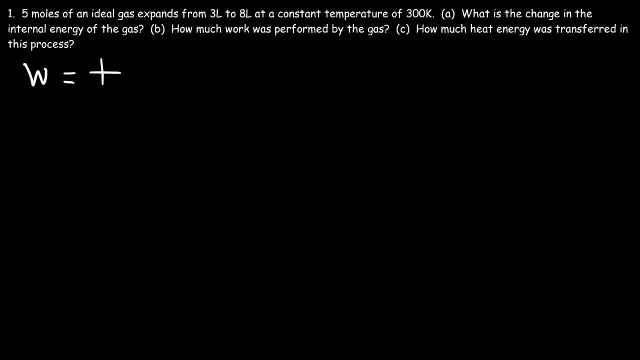 So work is done by the gas. Now how can we calculate how much work was performed For an isothermal process? this is the formula that you need. W is equal to nRT times the natural log of the final volume divided by the initial volume. 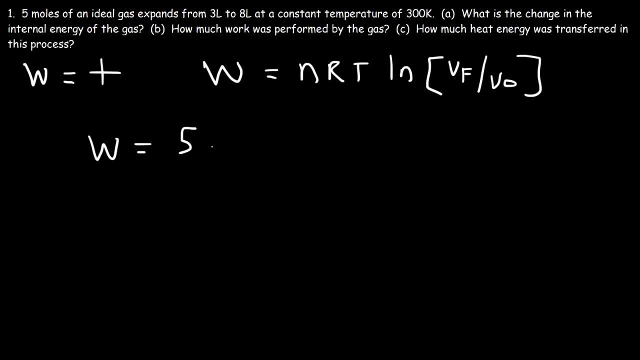 So in this example we have 5 moles. R is 8.3145.. And the temperature is 300 Kelvin. And then it's going to be the natural log of the final volume, which is 8 liters divided by the original volume of 3 liters. 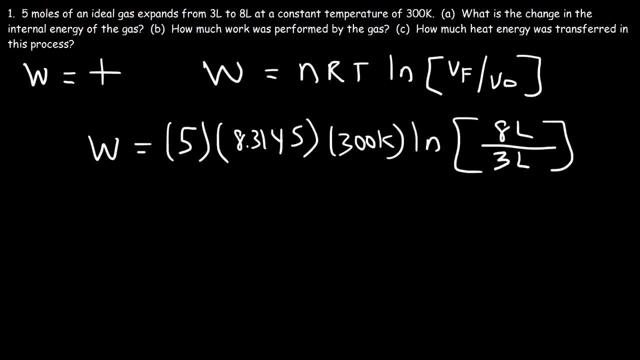 So go ahead and type this in. So W is equal to 12,233 joules. Round it to the nearest whole number. So that's it for part B. Now part C: How much heat energy was transferred in this process? Now we know that delta U is equal to Q minus W. 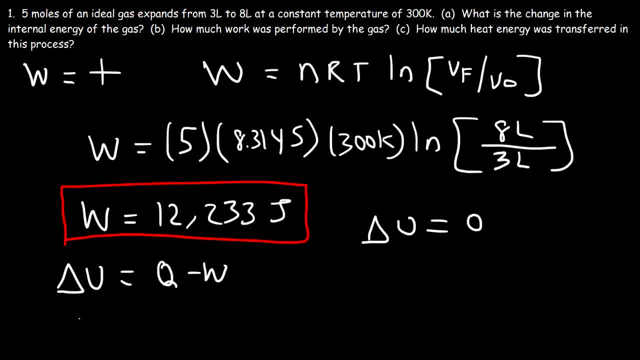 And for an isothermal process delta U is zero. So zero is equal to Q minus W. So if we add W to both sides, then the work performed by the gas is also equal to the heat energy transferred into or out of the gas. 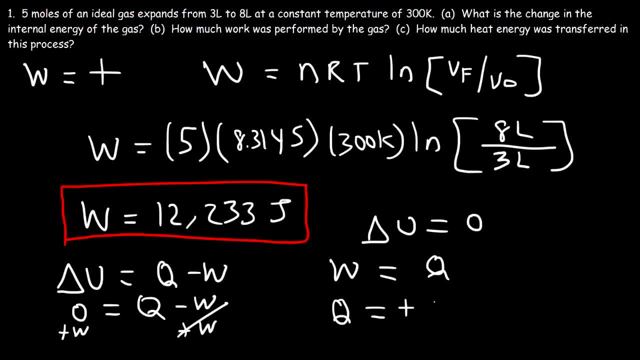 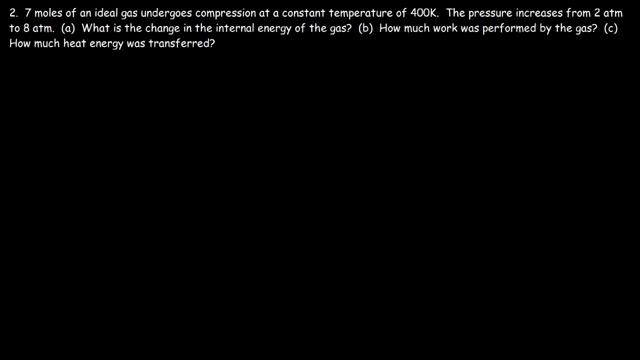 So in this case Q is positive: 12,232 joules. Because Q is positive, that means that heat energy flowed into the gas, causing it to expand at constant temperature. Number two: Seven moles of an ideal gas undergoes compression at a constant temperature of 400 Kelvin. 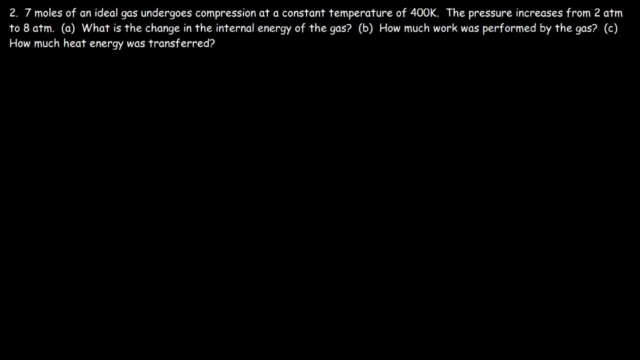 The pressure increases from 2 atm to 8 atm. What is the change in the internal energy of the gas? So we're still dealing with an isothermal process. The temperature is constant, So delta U is still equal to zero. So that's the answer for part A. 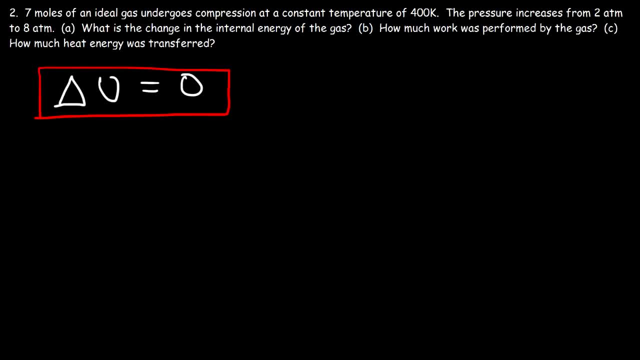 Part B, How much work was performed by the gas. Now, this time the pressure is changing at constant temperature. And the last problem: the volume was changing at constant temperature. So the formula we need is this equation: W is going to equal nRT times the natural log of the initial pressure divided by the final pressure. 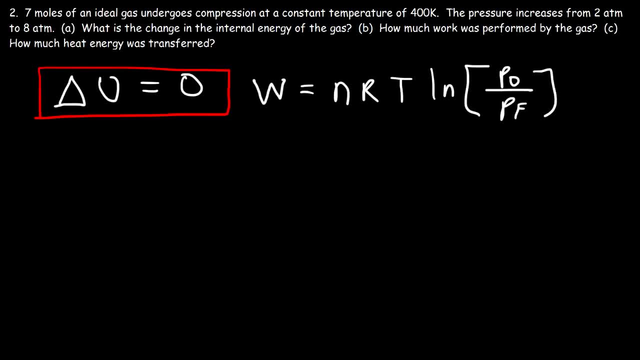 In the other problem it was the final volume over the initial volume. So let's plug in everything into this equation. So n is 7 moles, R is 8.3145 joules per mole per Kelvin And the temperature is 400 Kelvin. 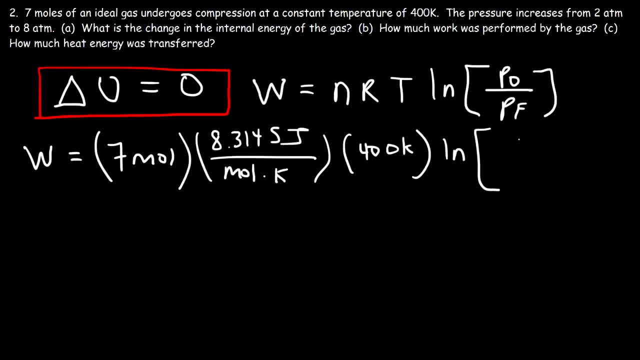 And then let's multiply by the natural log of the initial pressure, which is 2 atm, divided by the final pressure, which is 8 atm, So we can see that the unit moles will cancel. We could cancel Kelvin, And also the unit atm will cancel, leaving behind the unit joules. 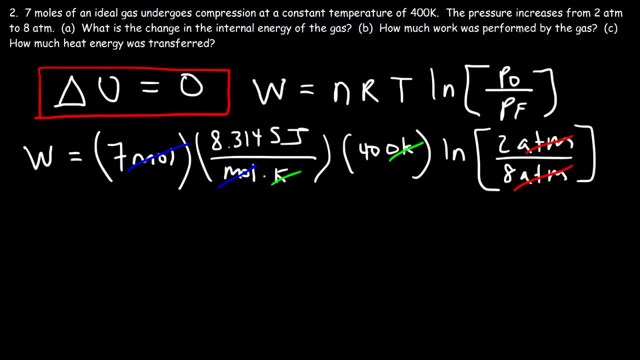 So W is negative 32,274 joules Now, because the gas is undergoing compression, which means that in order to increase the pressure, the volume has to decrease, And so the work done is negative. And the last problem: the gas was undergoing expansion. 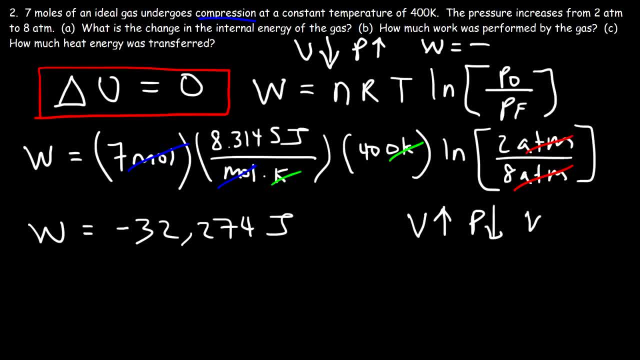 As the volume increases, the pressure decreases, And so the work performed is positive. So this is the answer to Part B. Now for Part C: how much heat energy was transferred? We know, for an isothermal process Q is equal to W. 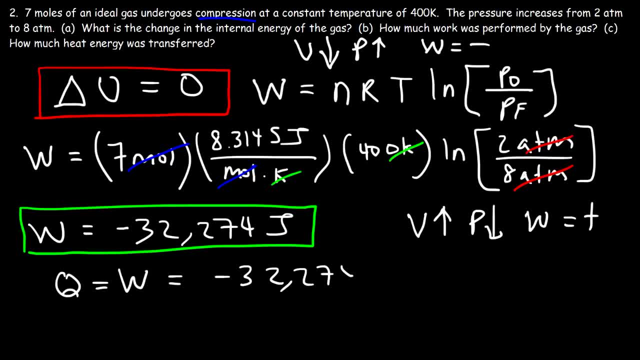 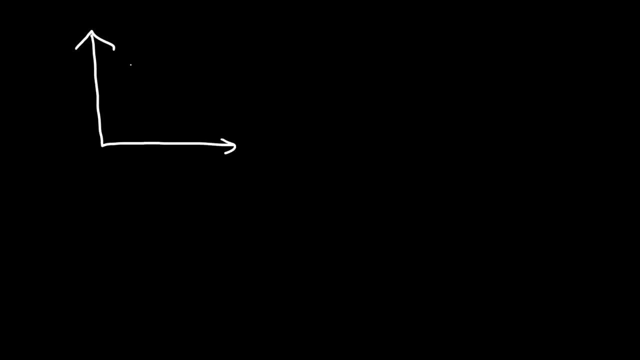 So Q is also negative, 32,274 joules. And because Q is negative, that means that heat flowed out of the gas as the gas was being compressed. Now let's talk about the PV diagrams for an isothermal process. So we have pressure on the y-axis and volume on the x-axis. 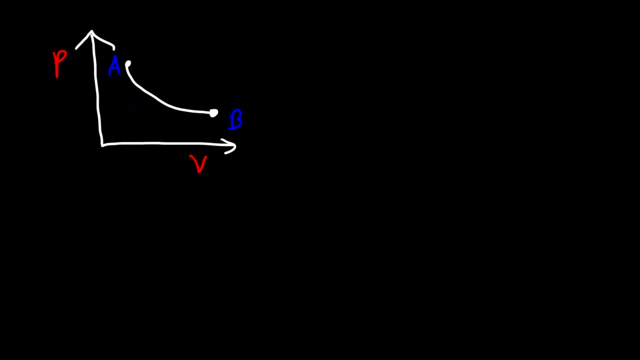 And let's go from A to B. So as we travel in this direction, notice that the volume is increasing and the pressure is decreasing, And as the gas undergoes expansion, the work performed by the gas is positive. Alternatively, let's say, if we travel from C to D. 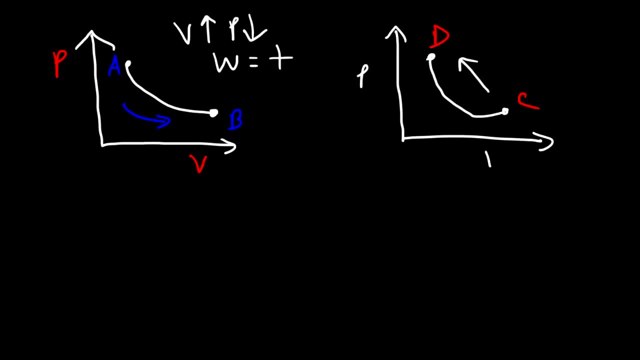 So we're going that way. As we travel from C to D, the volume is decreasing, The pressure is increasing, And so the gas is undergoing compression, and the work performed is negative. Now, to calculate the work done, it's equal to the area under the curve. 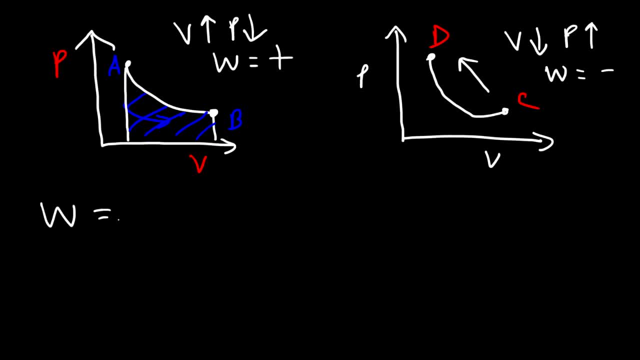 And to calculate the area under the curve you need to use calculus. Now, work is equal to pressure times, change in volume. if you have an isobaric process- But we don't have an isobaric process- However, work is still equal to pressure times, volume. 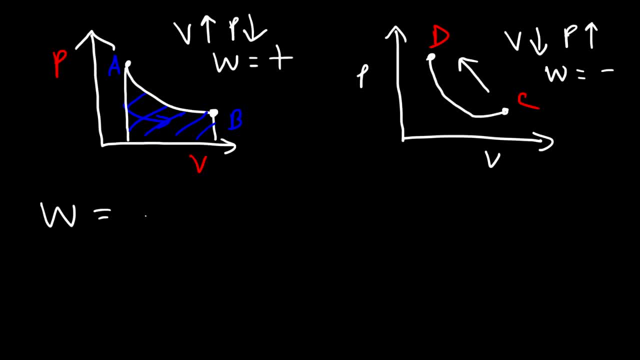 but for the area under that curve. So the formula that we need is this equation: It's going to be pressure times the change in volume, or dv, from V1 to V2.. So at point A, this is going to be V1.. 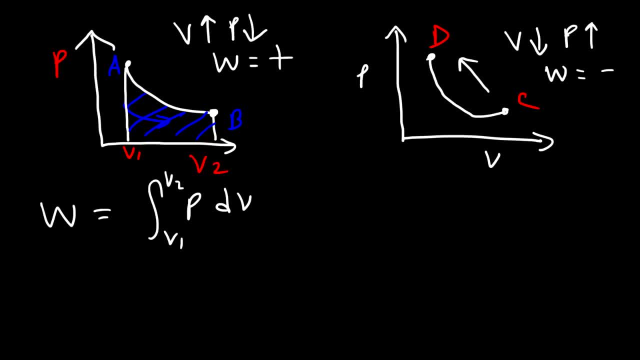 At point B, V2.. Now, based on the ideal gas law equation, we know that PV is equal to nRT. So, solving for P, the pressure is nRT divided by V. So I'm going to replace P with that. So that's nRT over V times dV. 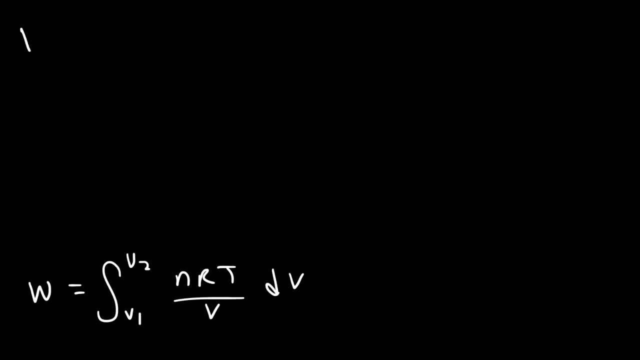 Now nRT is a constant, so I'm going to move that to the front. So W is going to be nRT integration from V1 to V2, 1 over V, dV, Now the antiderivative of 1 over x, dx. 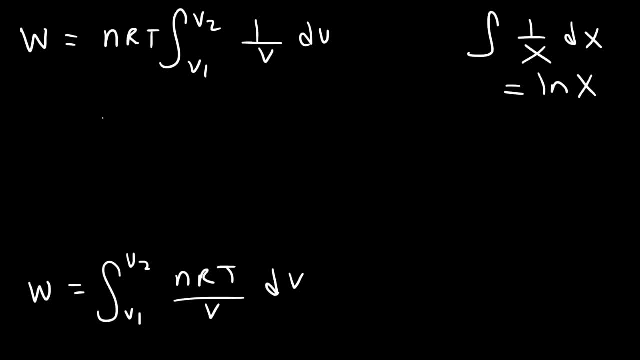 is the natural log of x. So for 1 over V, dV, it's going to equal the natural log of V, evaluated from V1 to V2.. So first we've got to plug in V2, which you can describe it as being V final.